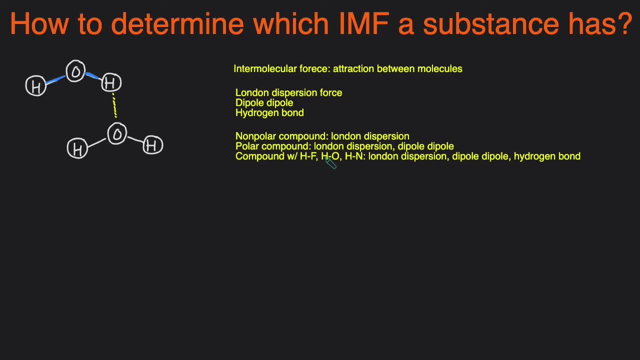 if you have a compound with H that's directly attached to F, H directly attached to O or H directly attached to N, then we'll have all three. We'll have London dispersion, dipole-dipole and hydrogen bonding. So everything, all compounds, have London dispersion. If it's polar, it'll also. 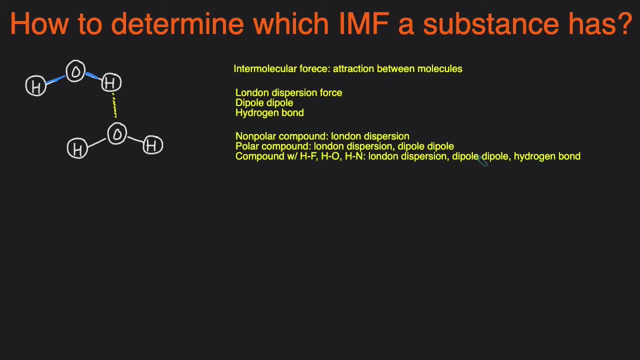 have dipole-dipole, And then if it has HF, HO or HN, then it'll have dipole-dipole and hydrogen bond. So let's take a look at some example problems and apply these rules. In this problem we have to determine what IMFs are present in the following substances. The first: 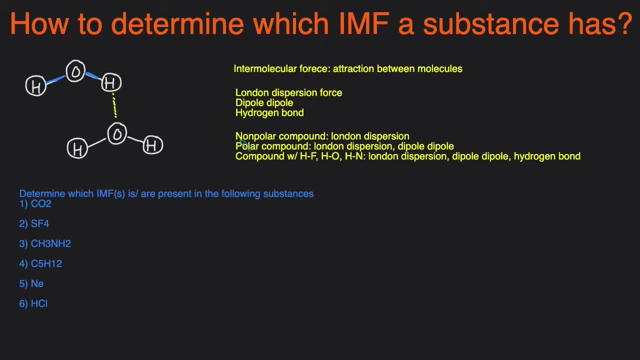 substance is carbon dioxide. To do this, we first have to determine if the compound is polar or nonpolar, And to do that you have to draw the Lewis structure. So I'm just going to draw the Lewis structure to save time. but if you're having trouble drawing the Lewis structure, check out the. 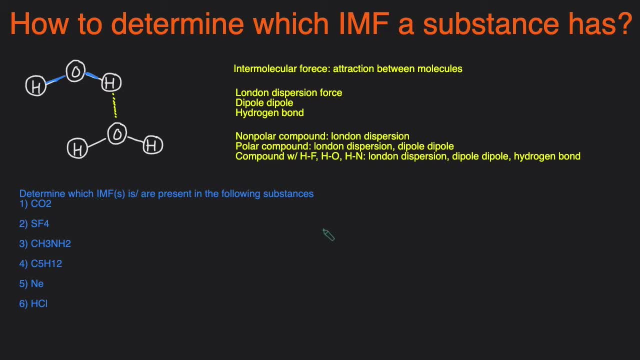 video in the description below where I go over that in detail. The Lewis structure for carbon dioxide looks like this: We'll have C with double bond and each of the Os have two lone pairs. Then we have to check whether this compound is polar or nonpolar, And to do that we can just use a quick checklist. 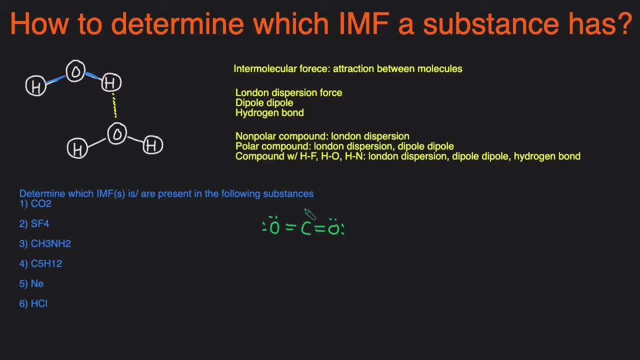 I have a video where I go over this in detail, but for the sake of saving time, I'm going to type out this checklist right here. So, the compound being nonpolarif, the central atom, the middle atom, has no lone pairs and all the atoms surrounding the central atom are the same. You can see, carbon meets criteria number one, because carbon doesn't have any lone pairs on it and it's just less介 feels. If you do that, you'll also consider the remaining no bind compounds. I've mentionedika đ Π fries together, but I think there are some components we need to consider. but instead of store and 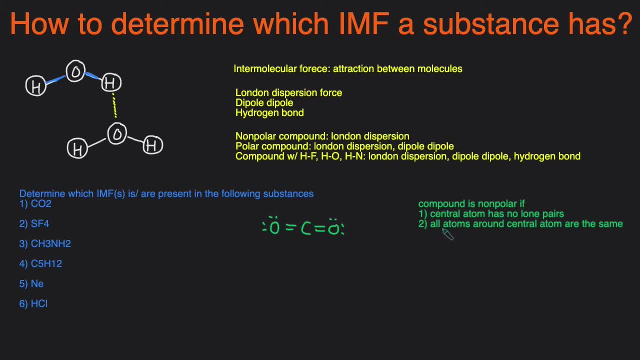 focus on the other components, reduce the量 slightly, And then, if we use this in small quantities, you'll 22 know that there also meets criteria number two, because both the surrounding atoms are oxygen. So that means that carbon dioxide will be nonpolar, and since it's nonpolar, it means that it only has London dispersion. 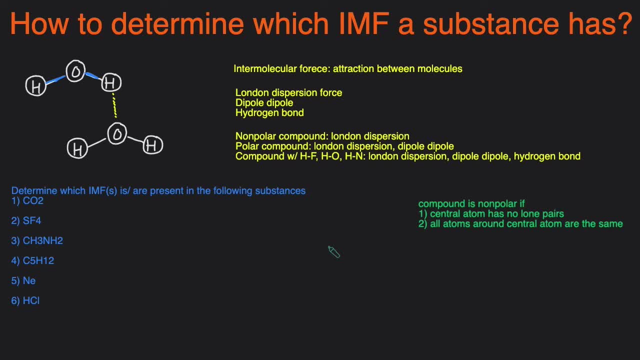 forces. So we'll start once again with the Lewis structure, and the Lewis structure SF4 looks as such. Then we need to determine whether this molecule is polar or nonpolar. so we use the checklist, we see if the central atom has any lone pairs, and S does have a lone pair on the central. 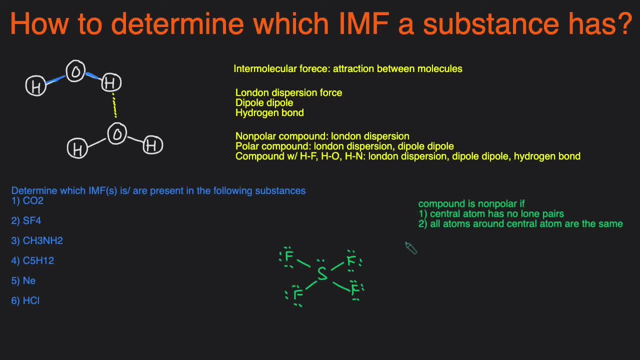 atom. so since it doesn't meet this first criteria, then I mean, this compound is going to be polar and since it's polar, it will have London dispersion forces and dipole. dipole. it doesn't have hydrogen bonding, because we don't see any HFHO or HN in this, in this compound. Okay, next. 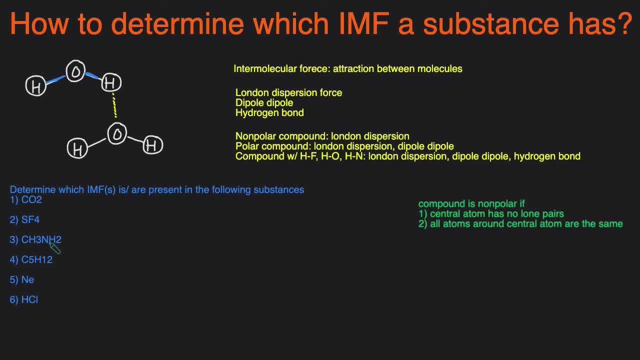 next sample: CH3, NH2. just right off the bat we see that there's an N and H right next to each other. so that means this compound meets. it has an NH, which means it's going to have London dispersion, dipole, dipole and hydrogen bond. So we need to determine whether this compound meets the HFHO or. 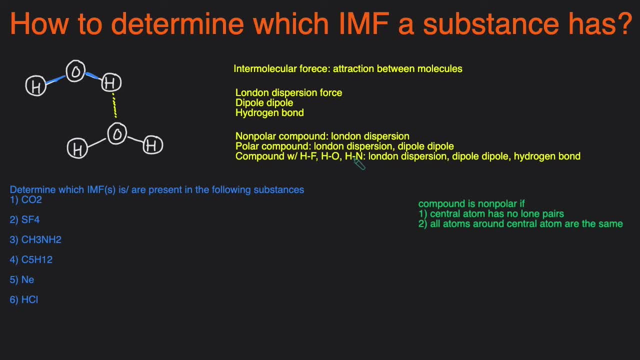 HN compound. So we need to determine whether this compound meets the HFHO or HN compound. So we need to determine whether this compound meets the HFHO or HN compound. So if you see HFHO or HN in the molecule, then you know it's going to have all three. Next example: C5H12. here's a. here's a neat. 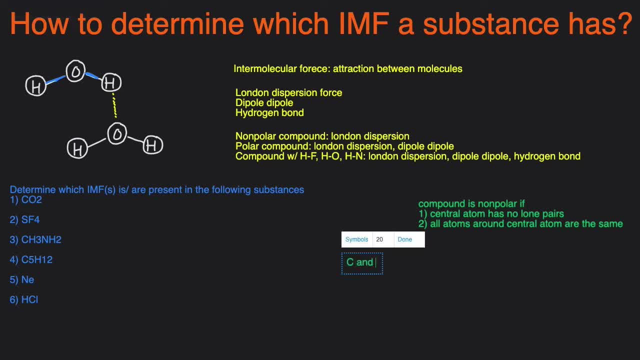 trick. so any compound containing carbon and hydrogen only is going to be nonpolar. So since C5H12 only has carbon hydrogen, it's going to be nonpolar, which means it will have London dispersion forces only. Other examples of this would be like C4H10,. 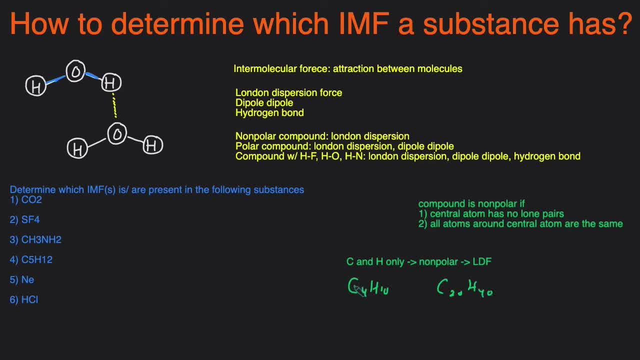 C20H4, H40. so any compound that just has carbon and hydrogen will be nonpolar, meaning it will only have London dispersion forces. Next example: Neon. this is a single atom, a single element. so if it's a single element then it has to be nonpolar, and since it's nonpolar, it will. 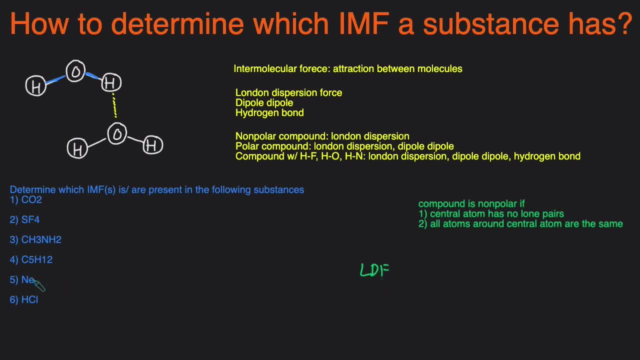 only have London dispersion forces, only for Neon. And then lastly, HCl. now we draw out the loose structure for HCl, it looks like this, and we know that Cl is more electronegative than H, which means that you're going to have a dipole moment pointing in this direction, and so that makes it polar. and if 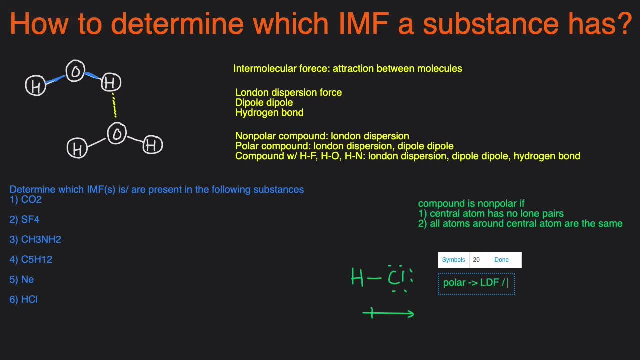 it's polar, it will have London dispersion forces and dipole-dipole, but it doesn't have hydrogen bonding because we don't see HF, HO or HN. And that's how you can determine what type of intermolecular force a substance has. The first step is just to draw the loose structure. then 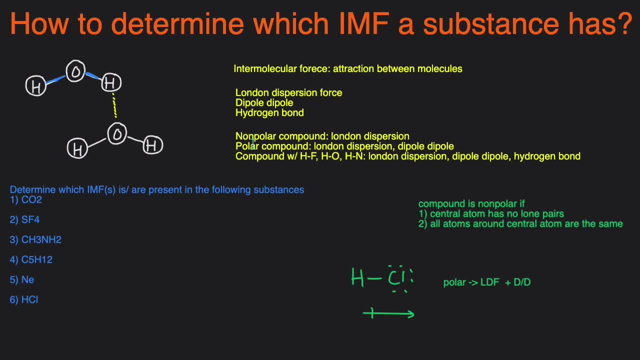 determine if it's polar or nonpolar. So once again I went over that pretty quickly to save time. but I have videos that teach you how to draw loose structures and determine if it's polar or nonpolar in detail. And if a compound has HF, HO or HN, then that means that's hydrogen bonding.